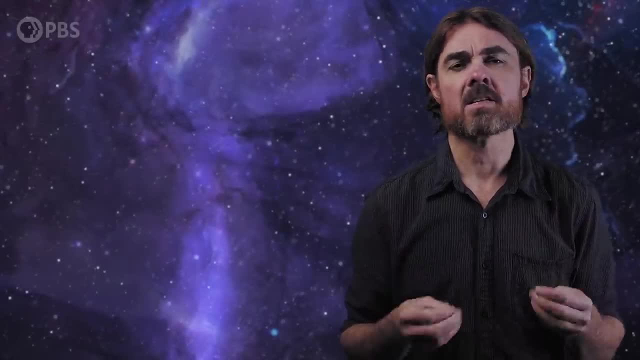 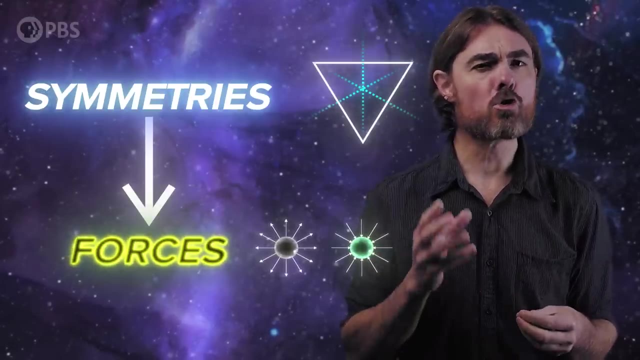 most important founding insights was the idea that the symmetries of nature give rise to the fundamental forces. Gage invariant says that the laws of physics are the laws of the universe. The laws of physics should not care how certain properties of the world are defined. 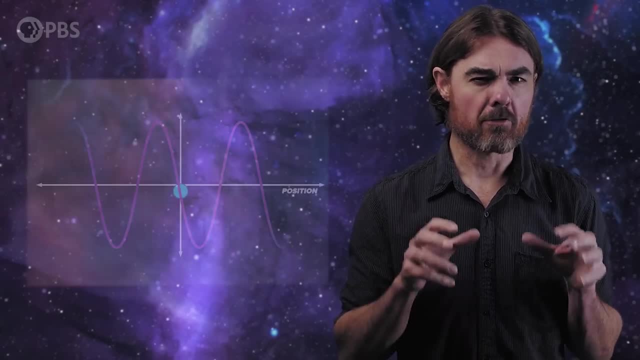 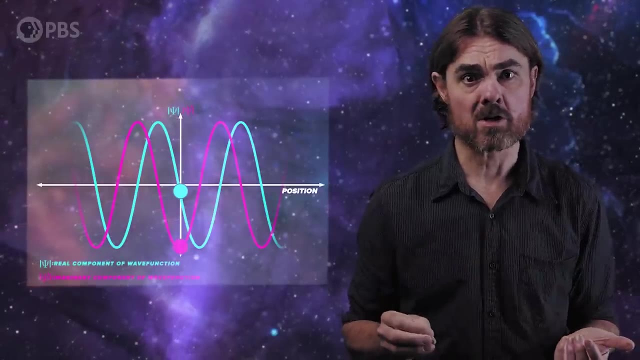 or measured. For example, if we insist that the phase of the quantum wave function is fundamentally unmeasurable, then we need to add a term to the Schrodinger equation to make that the case. That term turns out to be the electromagnetic field. So electromagnetism. 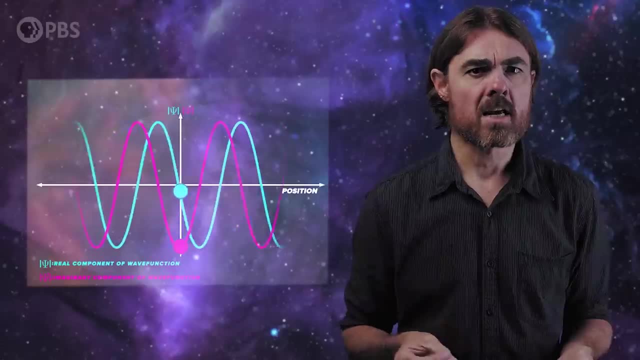 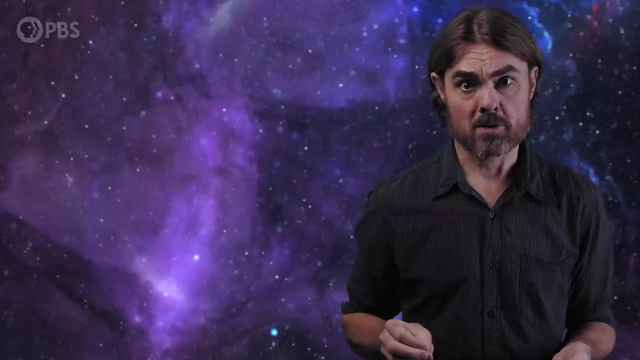 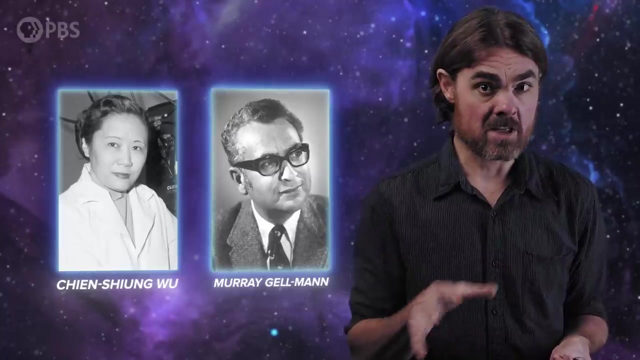 can be explained as being due to the fact that the universe has this particular, rather simple symmetry, which we call a U1 symmetry. That incredible success led many physicists over the decades to try to explain the other forces of nature in terms of gauge symmetries, And they succeeded. The weak interaction arises. 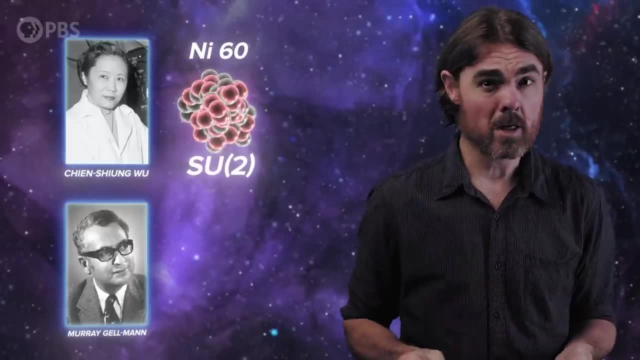 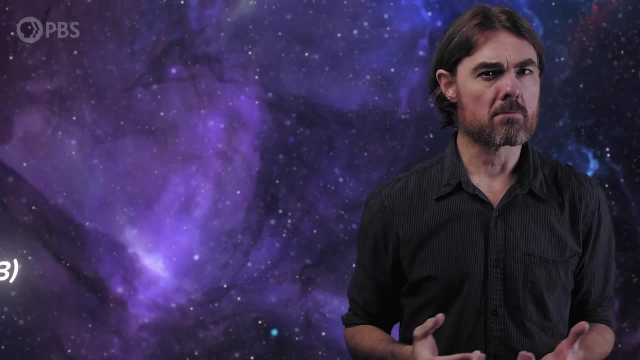 from a slightly more complicated SU symmetry, while the strong interaction is a consequence of the rather more complex SU. These symmetries also come from the fact that the wave function can be distorted in different ways that have no effect on the natural world. The way that the wave function can be distorted can be distorted in different ways that have 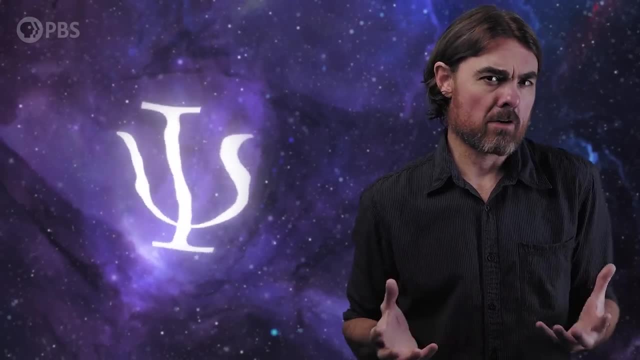 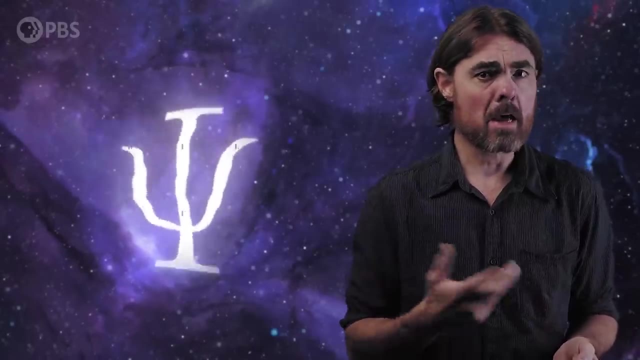 no effect on the laws of nature. It's just not as straightforward to say exactly what is being distorted as it is with the phase invariance of U1.. You may have noticed, though, that I skipped gravity. We're still working on that one. 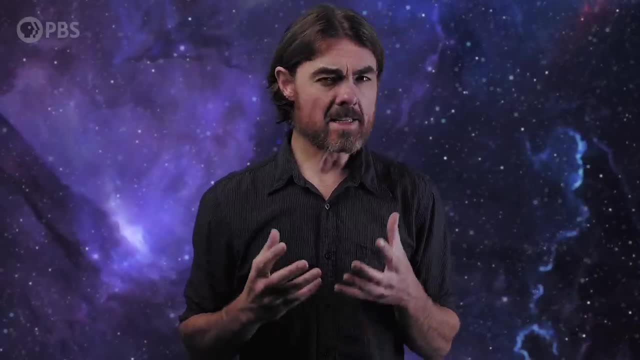 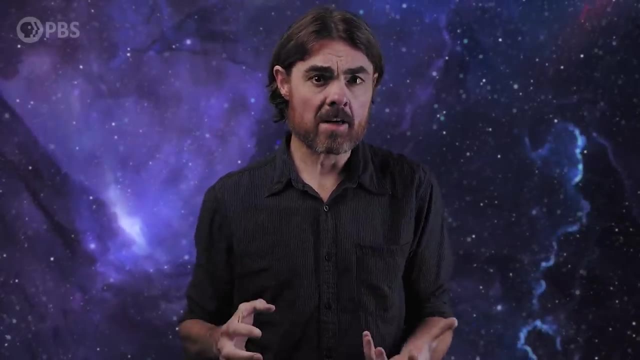 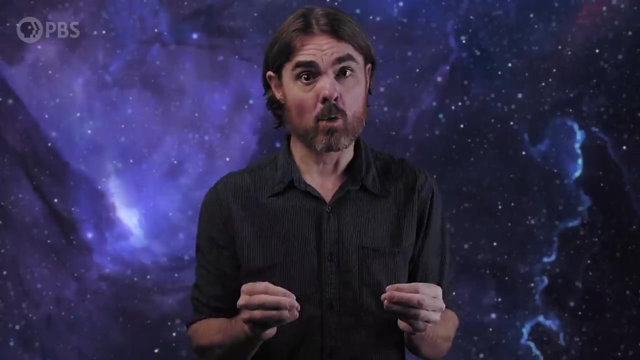 although it may have nothing to do with symmetries at all. It's a nice idea for all the forces of nature to arise from the same underlying mechanism, But how do you go from that to actual equations describing how the forces behave, And how do you wrap it all up in a single equation? that is the standard model Lagrangian. 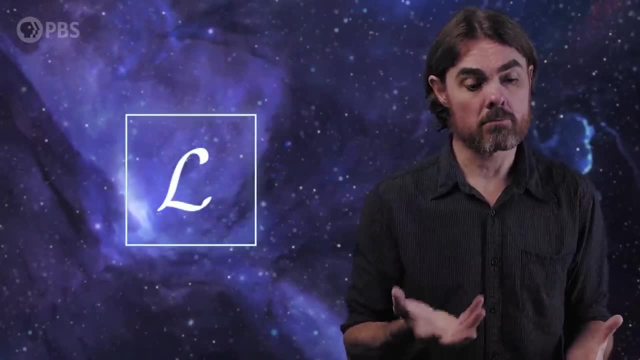 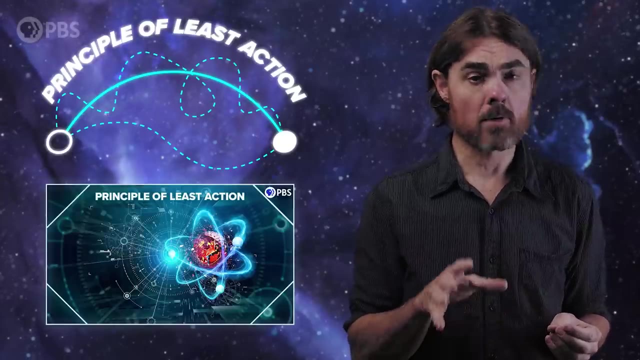 Well, the key is this Lagrangian thing, so let's talk about it. This is all possible due to an extremely powerful concept in physics called the principle of least action, which we've talked about in detail. It says that nature will always try. 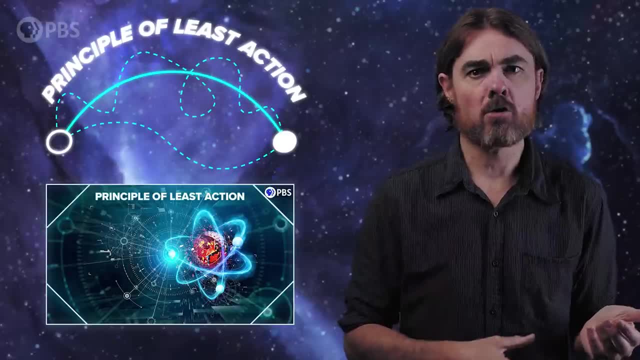 to follow the path that minimizes rate of change of a certain quantity called the action. This tendency can be used to figure out how pretty much anything can be changed in the world in a single equation. So let's talk about it for a moment. 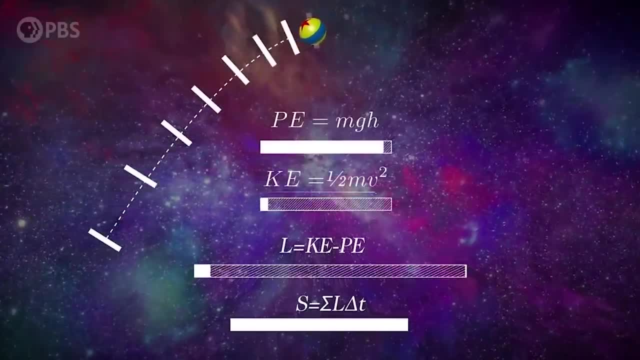 The principle of least action says that nature will always try to follow the path that minimizes rate of change of a certain quantity called the action. This tendency can be used to figure out how pretty much any process will play out, whether we're calculating the path traveled by a ball through the air. 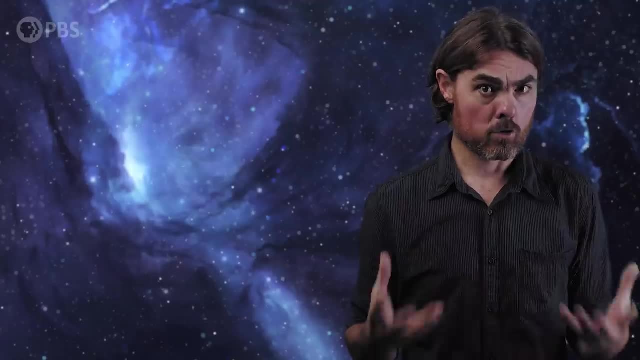 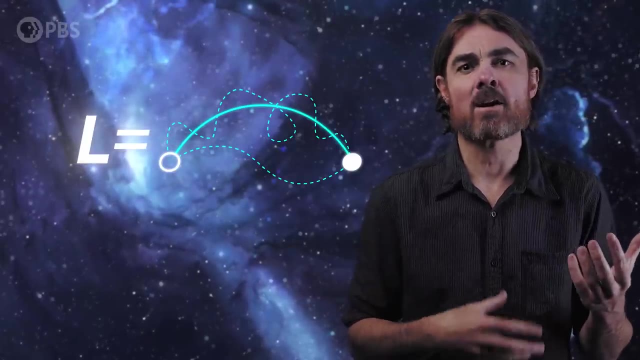 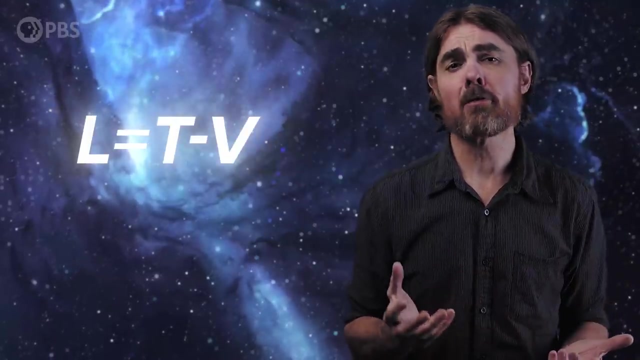 or the probability that two quantum particles will interact. The Lagrangian is the part of the action quantity that we actually work with. We can think of it as the distance an object or system travels through the space of all possible quantum states. For classical physics it simplifies to just kinetic energy minus. 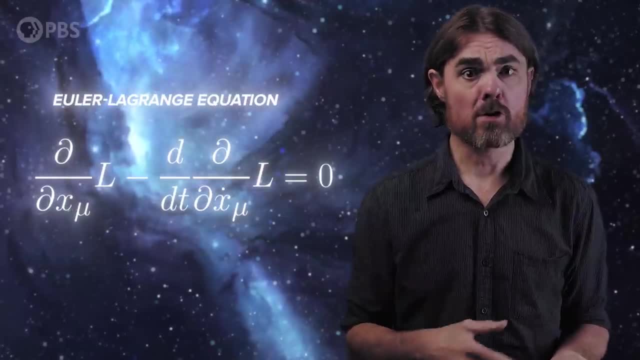 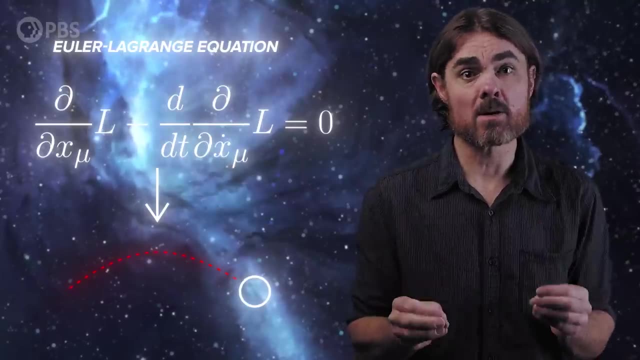 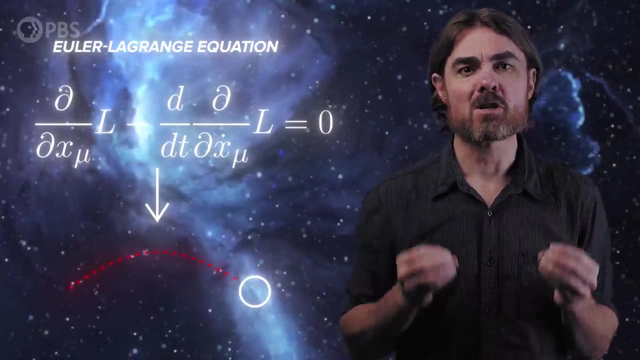 potential energy. If we plug the Lagrangian of a system into the Euler-Lagrange equation, then the result will be the equations describing how that system will move and change over time. There are other ways to get these equations of motion, but the Lagrangian is especially powerful. 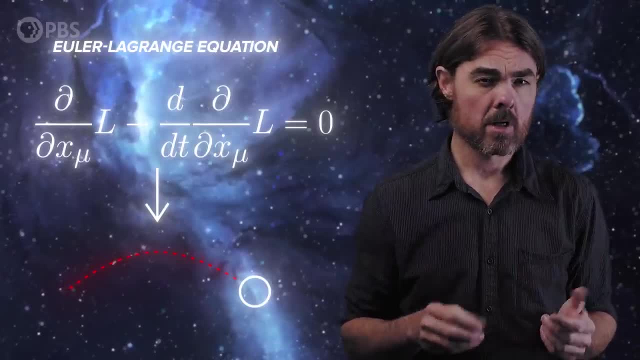 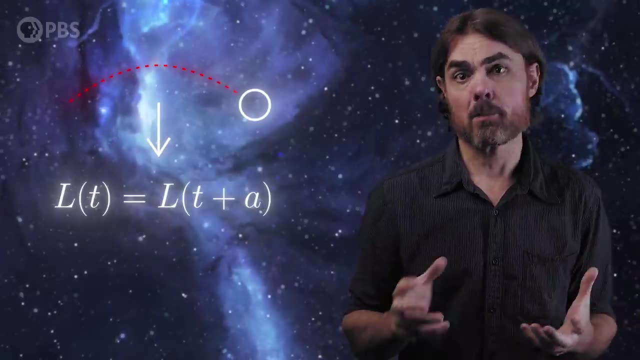 because of how it respects symmetries. If the system that we're studying has a certain symmetry, then the Lagrangian will have that symmetry too, And by applying the principle of least action to a Lagrangian with a condition of least action, the Lagrangian will be able 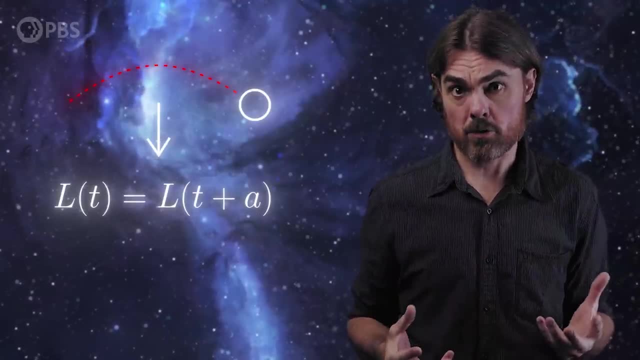 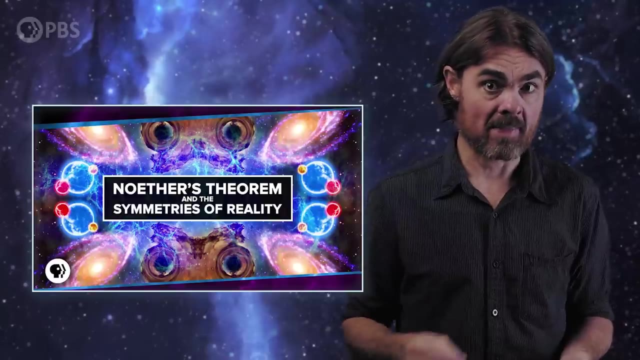 to move and change over time. The Lagrangian of a continuous symmetry will reveal the existence of a conserved quantity like energy or momentum. This is Noether's theorem, and we also have an episode about that. So it seems like it might be a good idea to figure out the Lagrangian for a wave function. 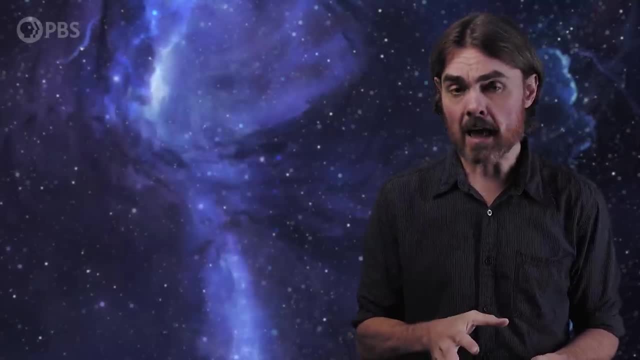 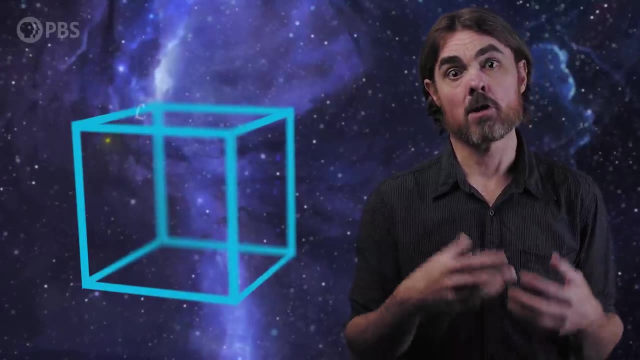 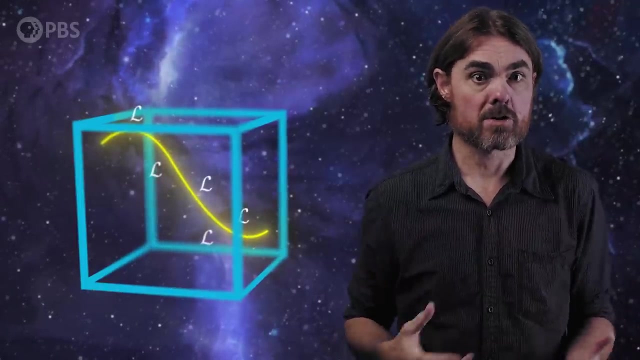 that has our symmetries of interest And that is exactly what the standard model Lagrangian is. I'm obliged to point out that this is technically not a Lagrangian, but rather a Lagrangian density, Which is like the building block of a Lagrangian, To get the real Lagrangian that describes. 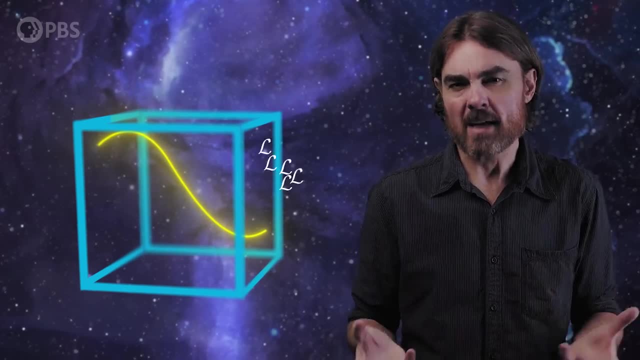 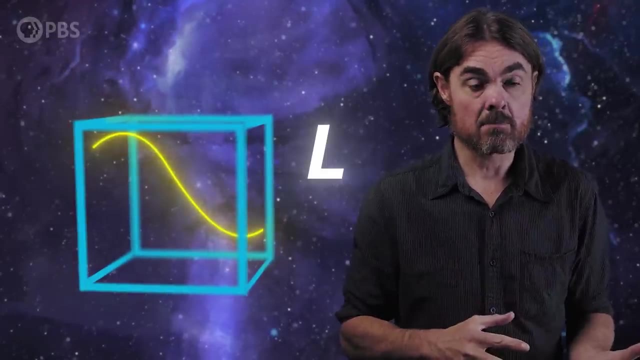 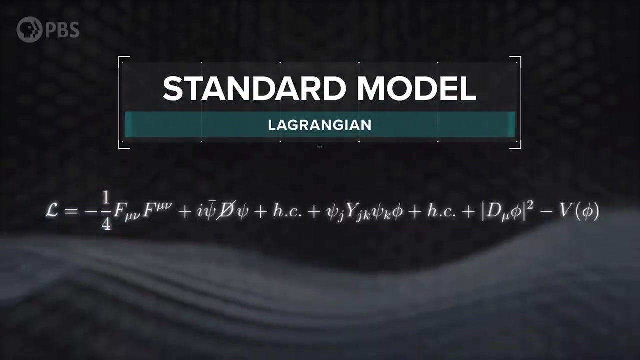 the behavior of particles in a certain volume. we have to add up infinitely many Lagrangian densities over that volume. although in practice everyone just calls Lagrangian densities Lagrangians, The standard model, Lagrangian, is complicated. It has several different terms that each account. 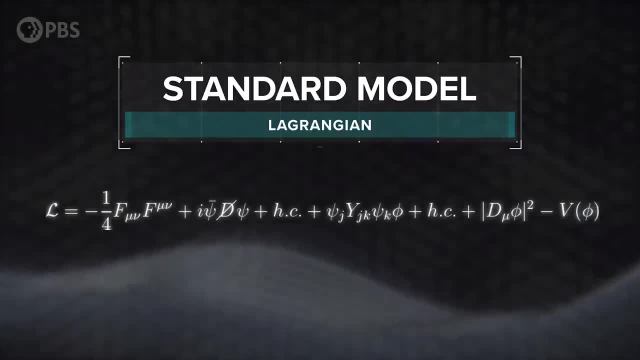 for different ways, that the particles of both matter and force interact, And each of these terms is actually a shambles. It's a shambles in the short hand for a lot of other stuff. Before we dive into what all of this means, let's go over what we have to describe. 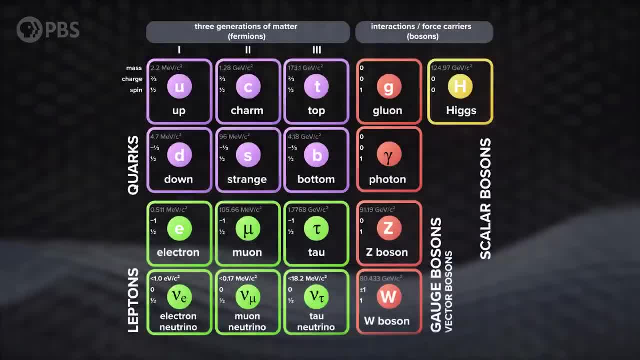 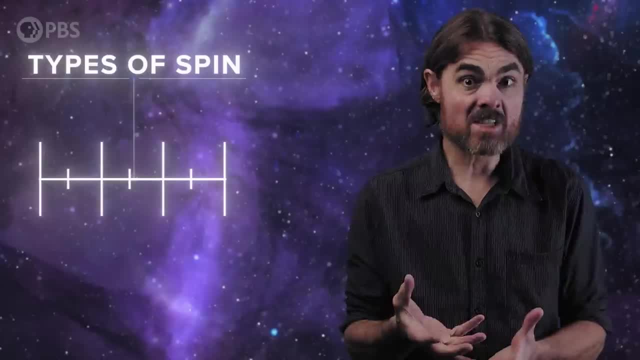 Namely the particles of the standard model and their interactions with each other. The symmetries I mentioned allow for particles to have two different types of spin. They can either have an integer amount of spin, like 1,, 2,, 3, or even 0. Or they can have 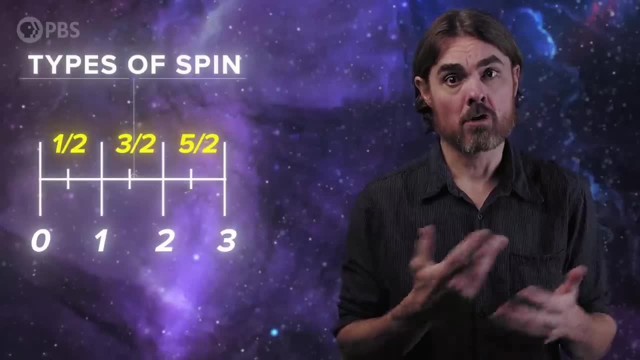 a half integer spin, like a half 3 on 2, 5 on 2.. It turns out that spin determines the speed of the particle. In this example, the spin of the particle is the speed of the particle. The spin determines what might be the most fundamental nature of a particle, whether 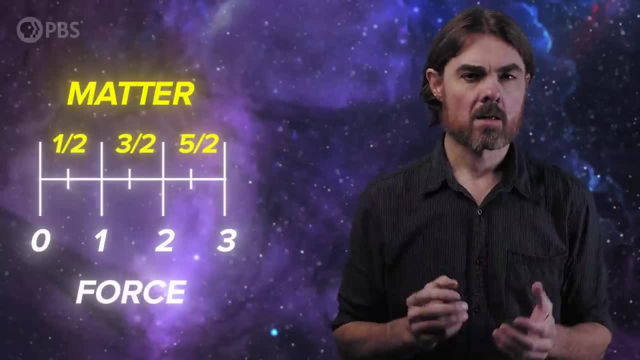 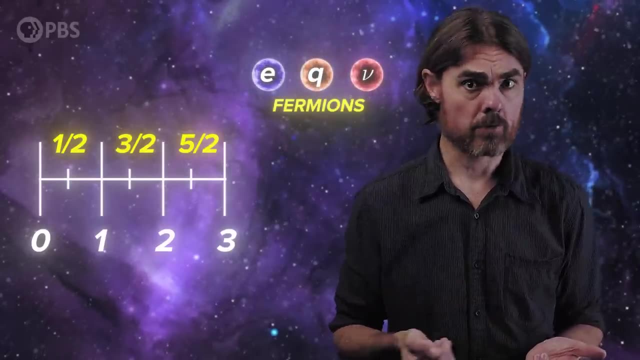 it represents matter or force. Particles with half integer spin are called fermions and they are stuff. Literally they are. what stuff is made of: Electrons, quarks, neutrinos. they are all just different kinds of fermion. 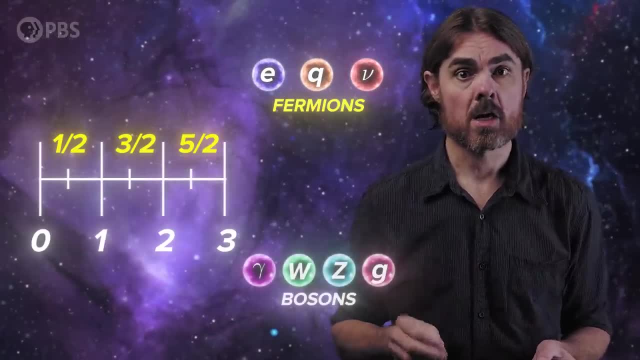 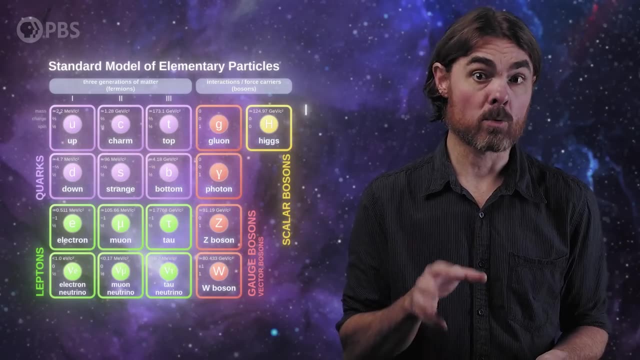 Meanwhile, particles with integer spin are called bosons. They transmit energy and momentum according to the symmetries of each force. Some parts of the standard model Lagrangian deal with bosons, other parts deal with fermions and still others, perhaps the most important. 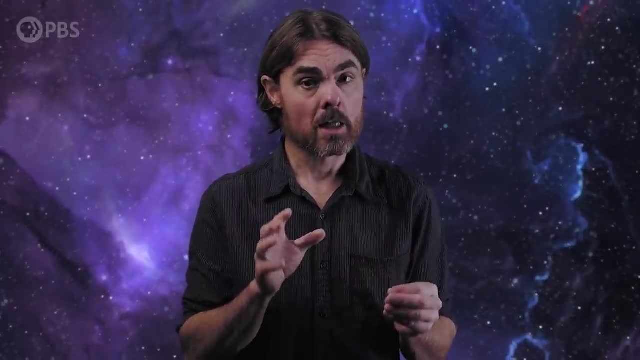 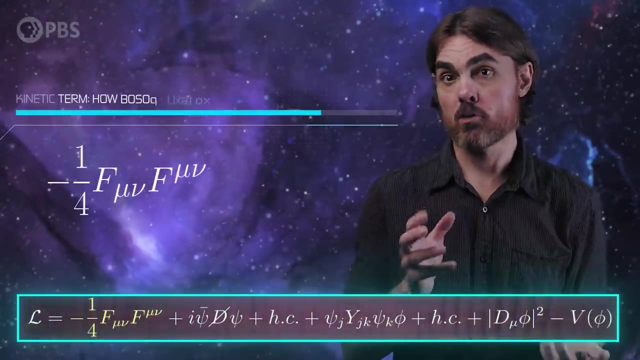 parts deal with the interactions between the two. So let's now take a tour through the standard model Lagrangian and see what it's all about. First, we have this term with the two F's. This is known as the kinetic term, and it. 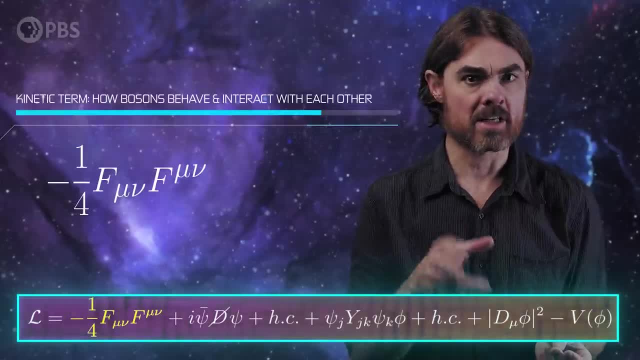 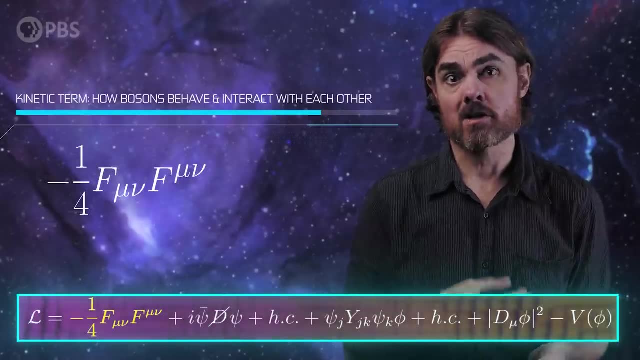 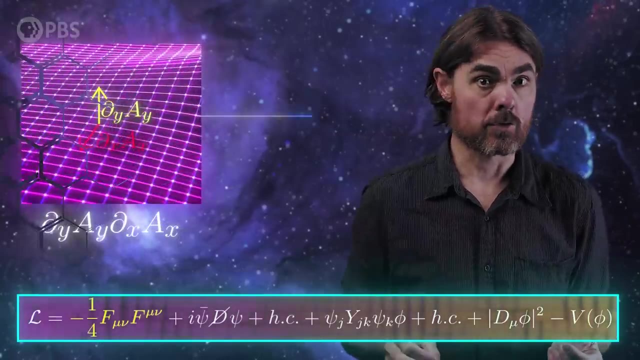 tells us how the bosons will behave and how they'll interact with each other. Alone, this describes a universe with no matter whatsoever. The F's are actually a shorthand for the separate interactions of each of the three quantum forces. First we have the photon field, which is usually represented with a capital-A. This 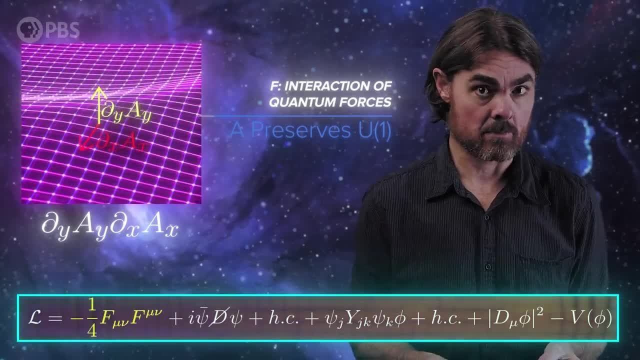 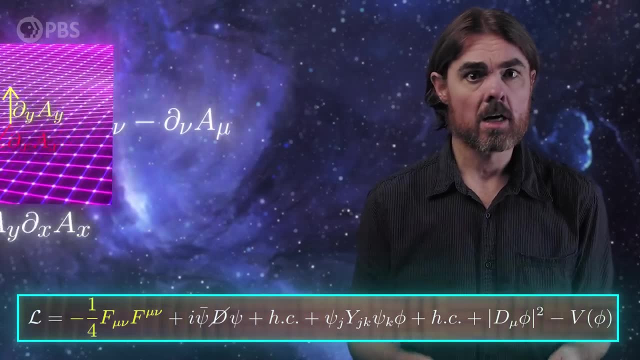 is the field that preserves the U1 symmetry of electromagnetism, And the kinetic term for photons is made up of the derivatives of the A field. In other words, this is like the energy of the photons as they change in space and time, And this is true for all the 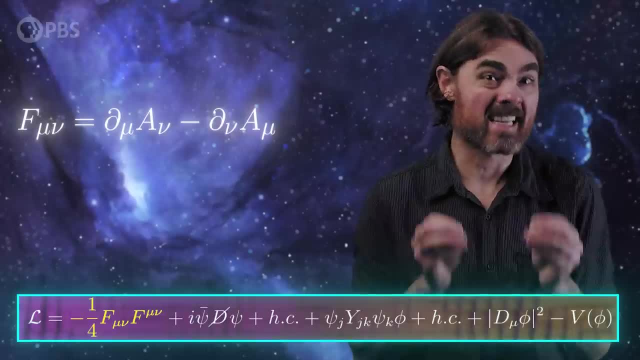 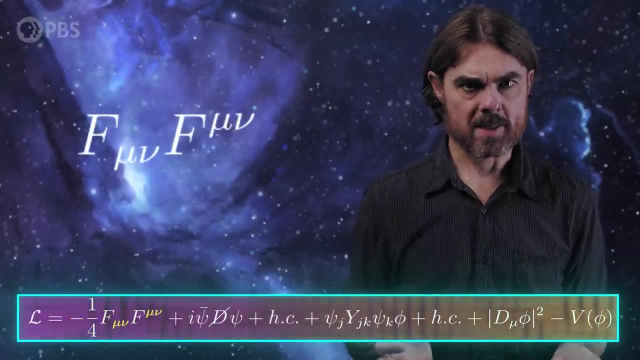 derivatives that we're going to see here. They are analogous to the kinetic energy of that object in every direction of space and time. This is where the mu and nu symbols come from. The kinetic energy of the field in one direction may depend on what is happening in the other. 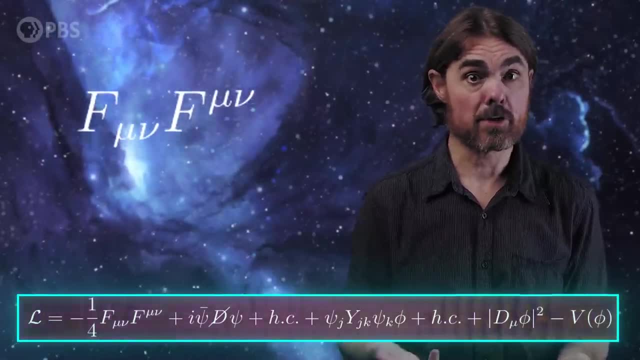 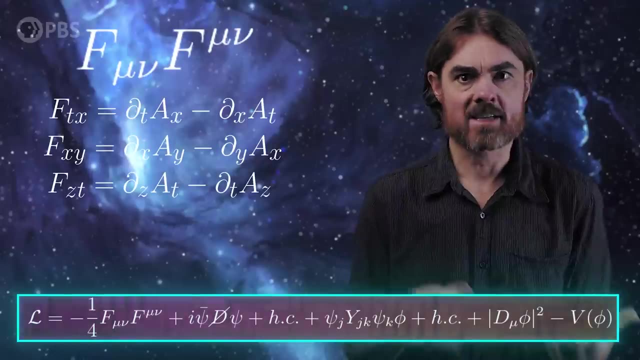 directions, which means we need to take a lot of derivatives of the field in every direction. Instead of writing each one, we just write these symbols, which basically mean: first do the x direction, then y, then z, then do t for time. 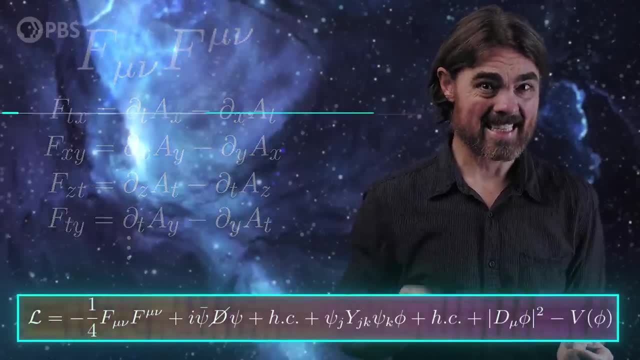 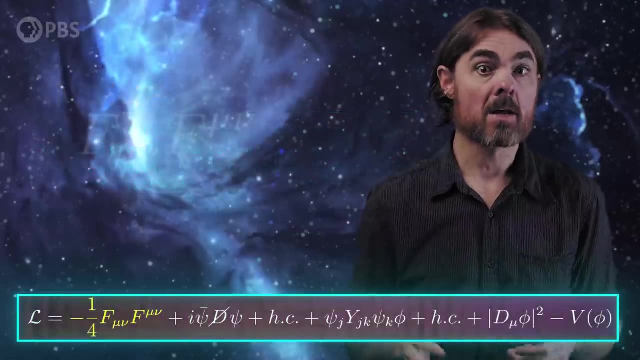 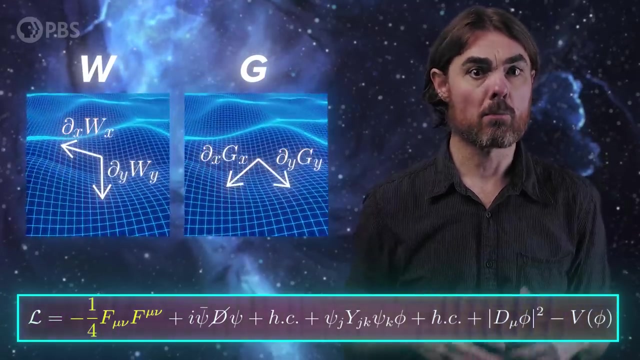 Indices are going to be a running theme here. Whenever you see indices, it means that whatever was written has to be repeated several times, depending on the dimensions of spacetime, the number of charges, the number of different particles, things like that. Next we do something similar for the fields of the other two forces. 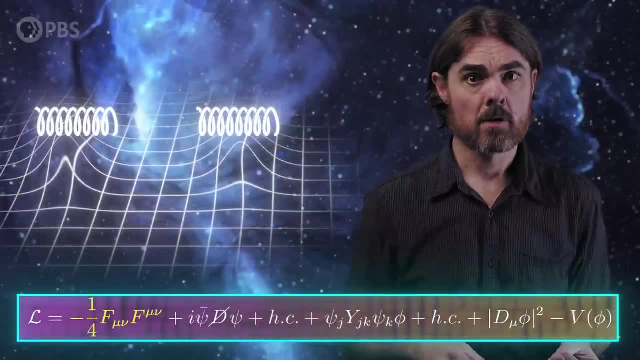 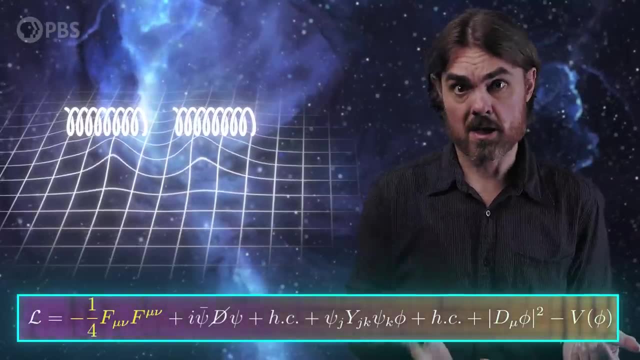 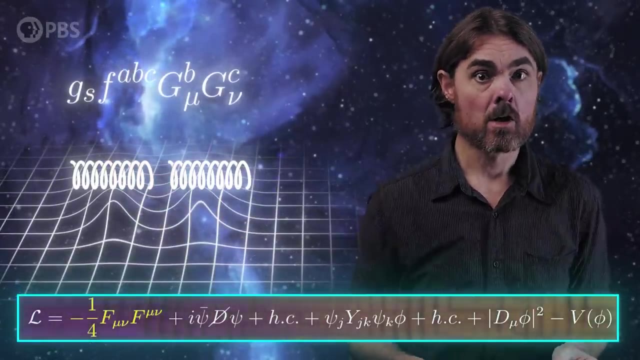 We also need their kinetic energy in every possible direction. Except if two photons come close, they'll just pass through each other, But if two, say gluons come close, they will interact. We need an extra term to describe the potential energy of that interaction which we add to. 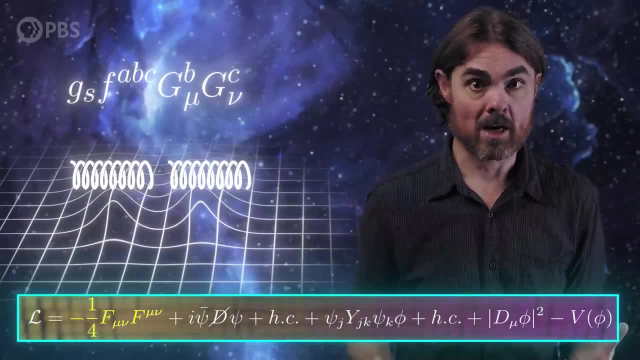 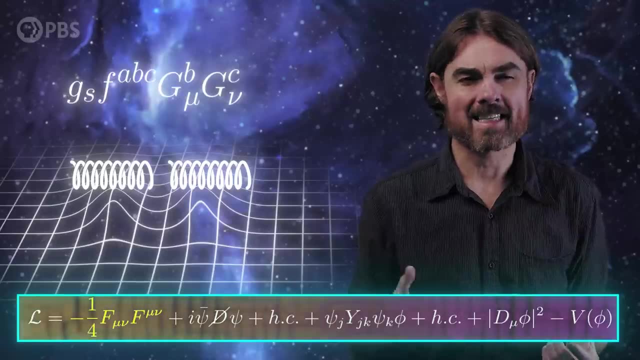 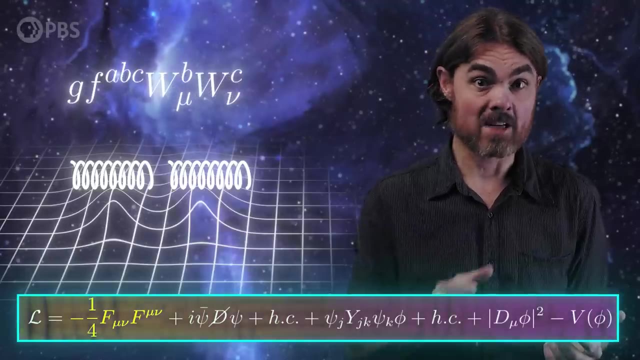 the kinetic term. Here we see a connection to the classical Lagrangian with its kinetic and potential energies. The many indices that you see here come from the complex symmetries of SU and account for all the different types of gluon. The bosons of the weak force get a term like this also, but its SU symmetry leads to different behavior. 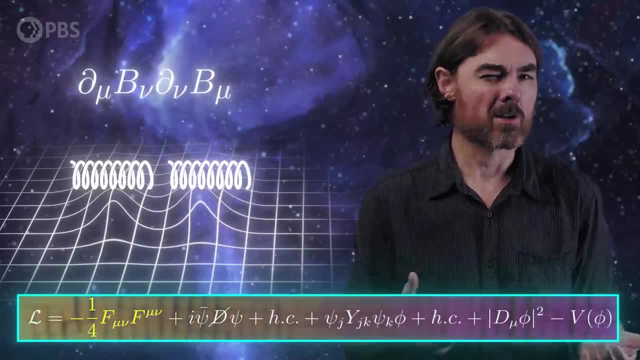 The weak force is the force of the weak force. The weak force is the force of the weak force. The weak force is the force of the weak force. The weak force also has a second kinetic term that looks a lot like electromagnetism. 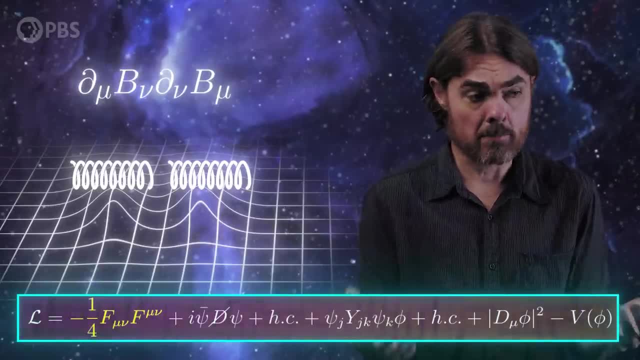 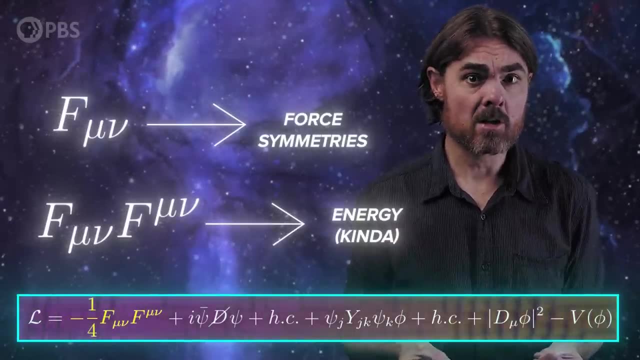 a consequence of the fact that the weak force and electromagnetism used to be components of the one force. These complicated kinetic terms are multiplied with themselves in a matrix multiplication because that turns them into the appropriate units of energy or something close to energy. 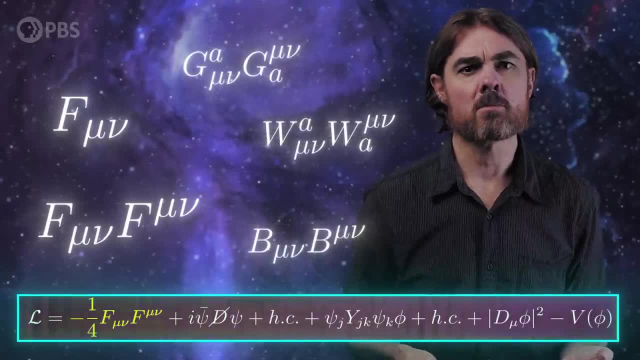 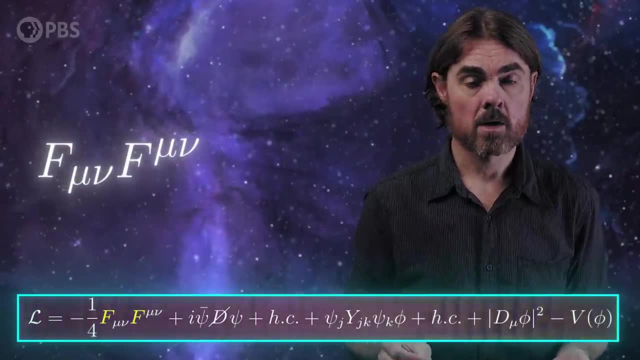 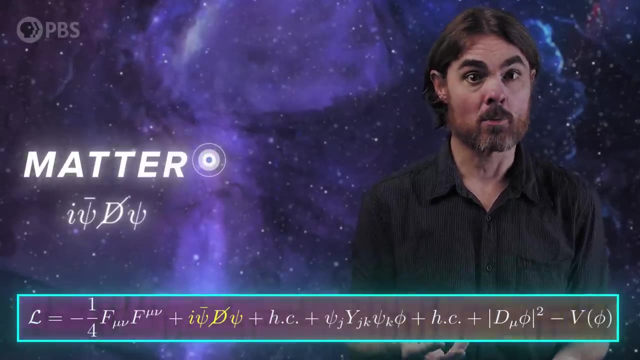 because that's what the Lagrangian needs. All these kinetic terms are summarized with the Fs representing the motion of the bosons and their interactions with each other. Okay, let's make the universe more interesting by introducing some matter. That's what the second term in the Lagrangian represents. 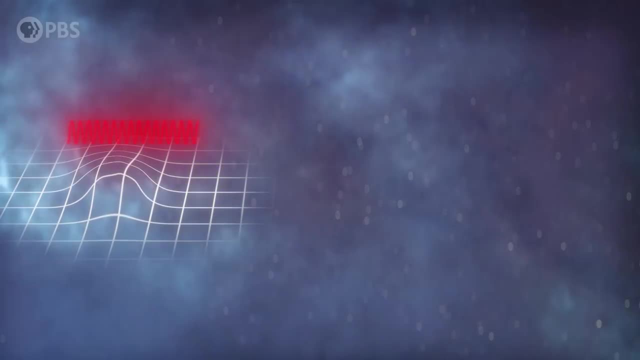 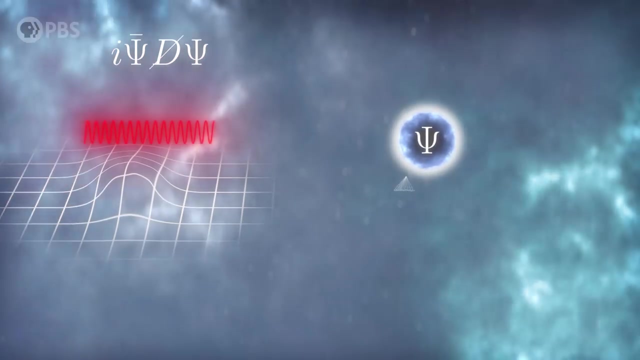 The psi is the wave function of the fermion fields. Strictly speaking, there are 12 fields for the 12 kinds of fermions that we've discovered so far, But again they're squished together into this one symbol. Let's look at this weird d thing. 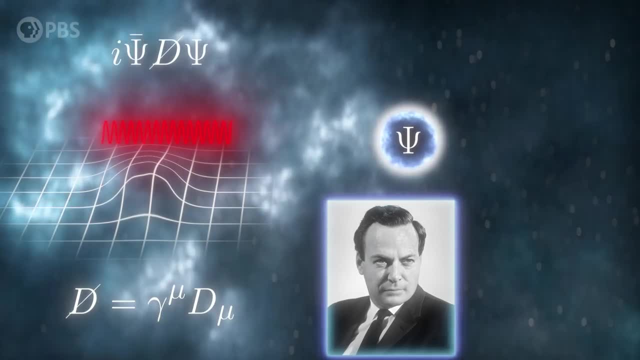 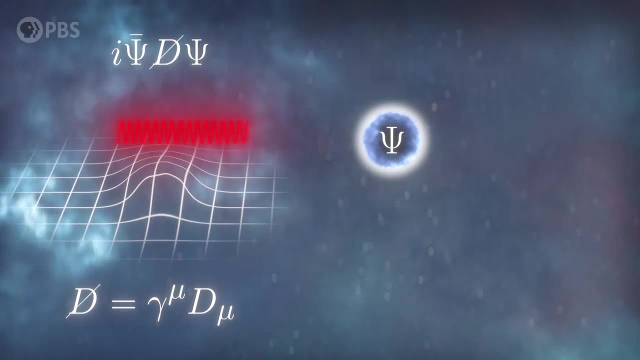 The slash is a shorthand that Richard Feynman came up with because he was tired of always having to write GAN. That's gamma d, Where gamma is a series of matrices to ensure that everything stays compliant with general relativity. The d itself is made of two parts. 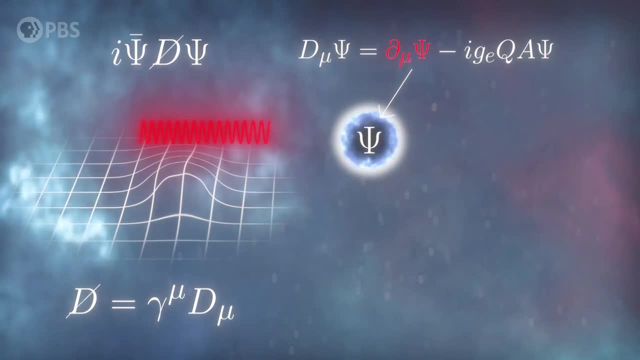 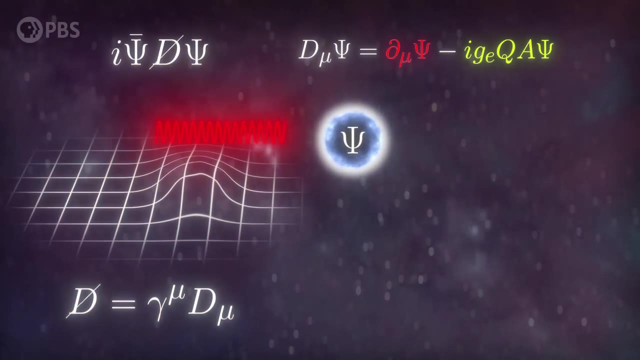 We have a derivative which, as we mentioned, tells us the energy of the field as it changes. But we also have this part with the field of the bosons. This tells us how fermions are going to interact with the fields that preserve the symmetries. 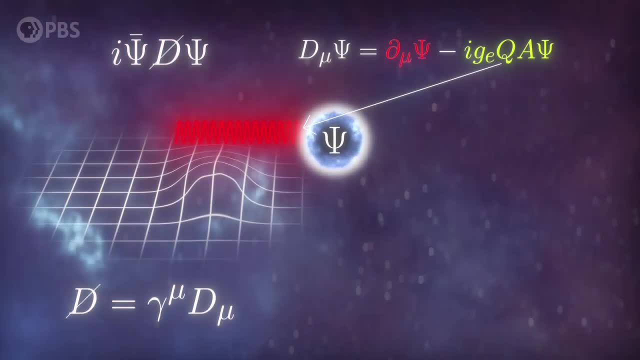 of nature. This is the piece that tells us how matter and the bosons interact. This is the piece that tells us how matter and the bosons interact. This is the piece that tells us how matter and the bosons interact and forces interact. 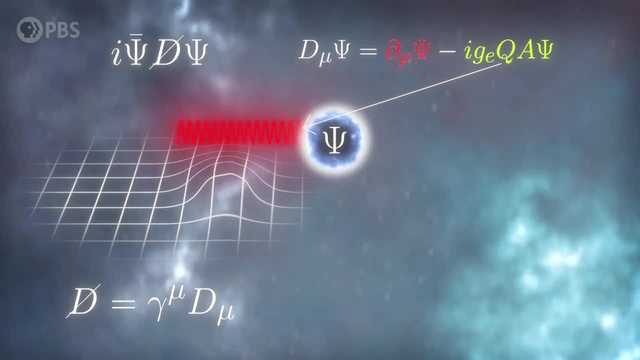 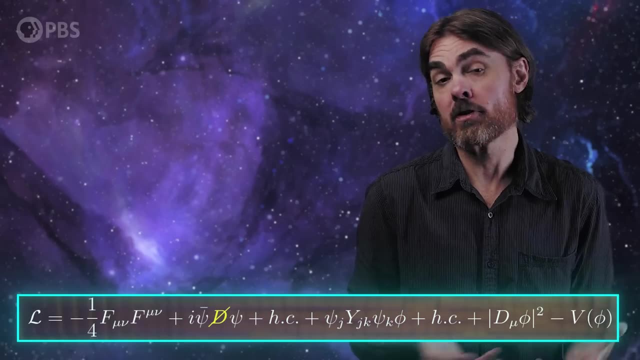 The part with the electromagnetic field is equivalent to the piece that was added to the Schrodinger equation to ensure phase invariance. And now we have to add the pieces for the other fields also. Here, each field is preceded by a new symbol. 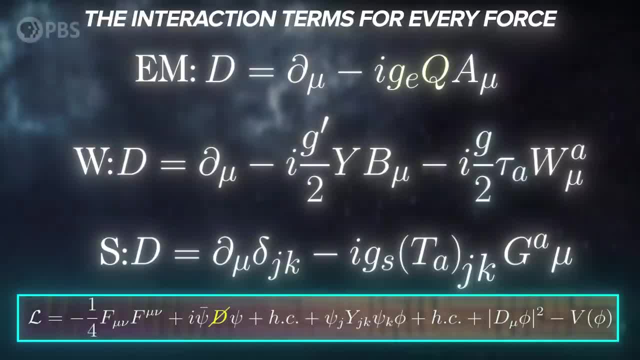 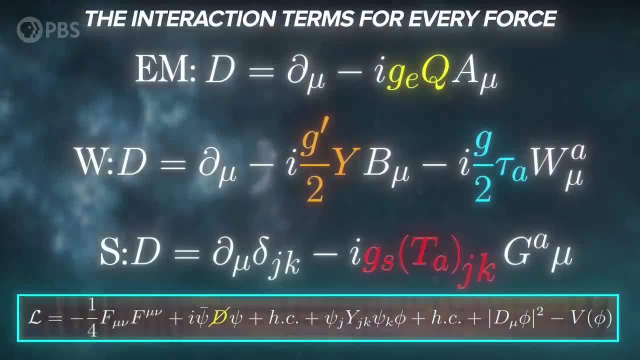 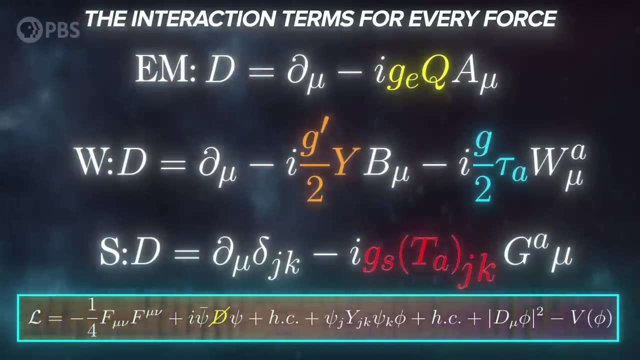 which represents the charge that the field interacts with. We have electric charge, isospin, hypercharge and color charge, And the more complex the symmetry, the more indices you need. Also, next to the charges are the coupling constants, which represent the strengths of each interaction. 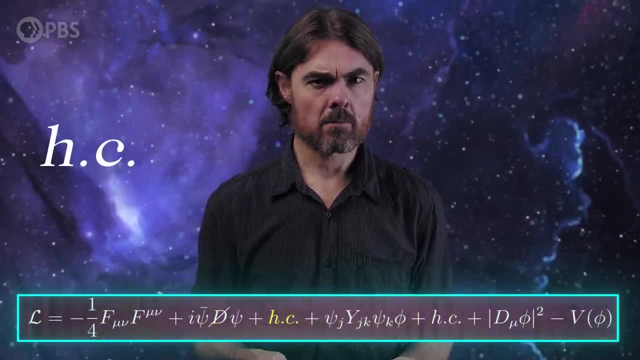 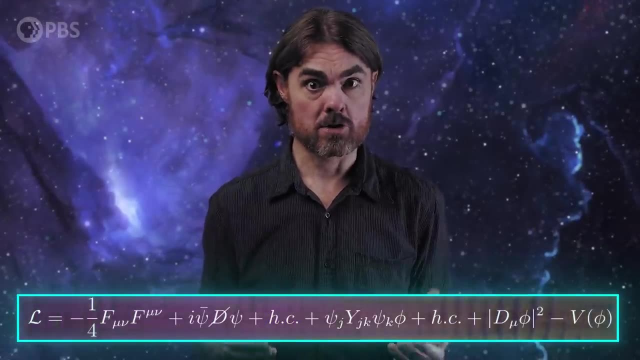 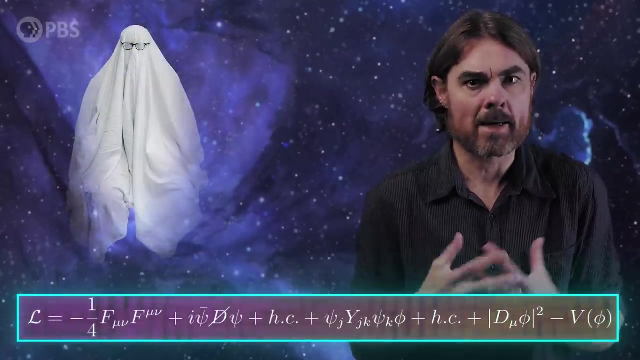 And here we have this hc thing. And well, I didn't want to scare you earlier, but this Lagrangian is haunted, It has ghosts. There are ghosts of particles that can't be measured and ghosts of infinities that make no sense. 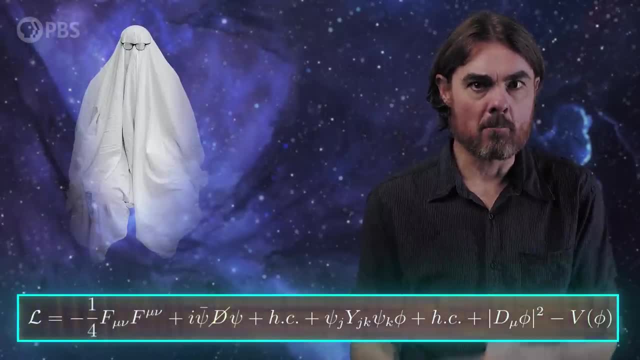 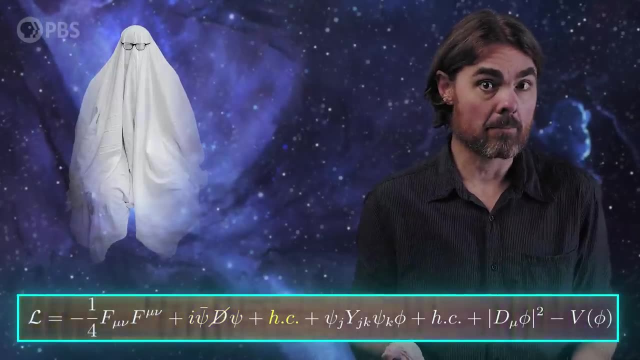 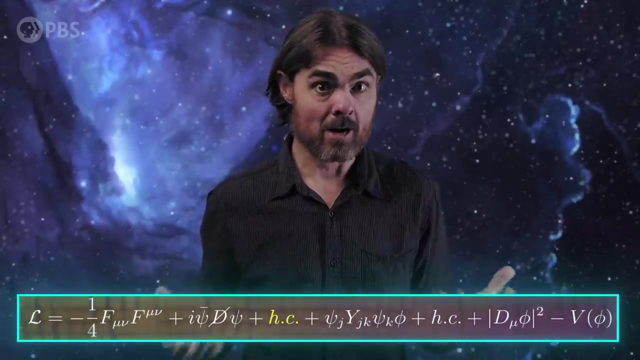 But it turns out that if you add a copy of the matter term, that you switch the sign in front of every imaginary number, all of the problematic ghosts cancel out. Now this process may sound a bit forced, and it kind of is. It would be nice to have a Lagrangian without ghosts. 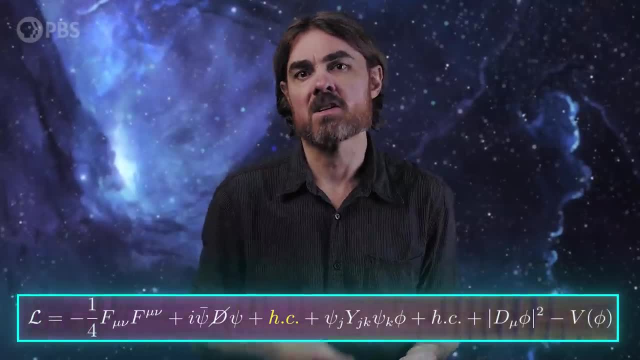 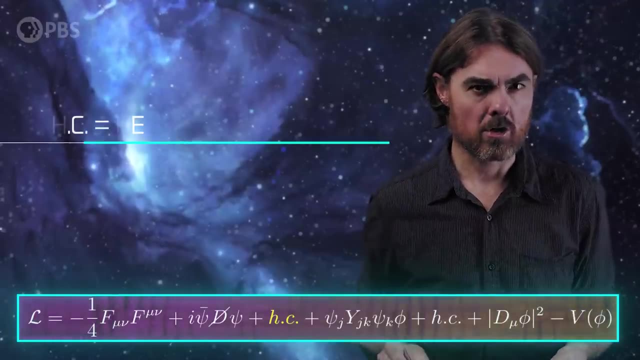 and perhaps one day we will, But until then, this process gives us an equation that describes nature very well. By the way, the hc stands for permission conjugate, which is the process of flipping the signs of the imaginary components, And it can also stand for: 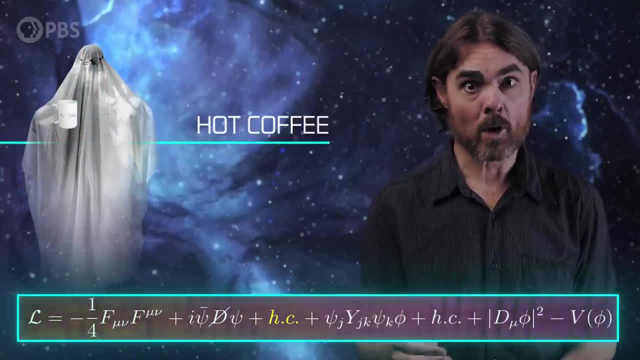 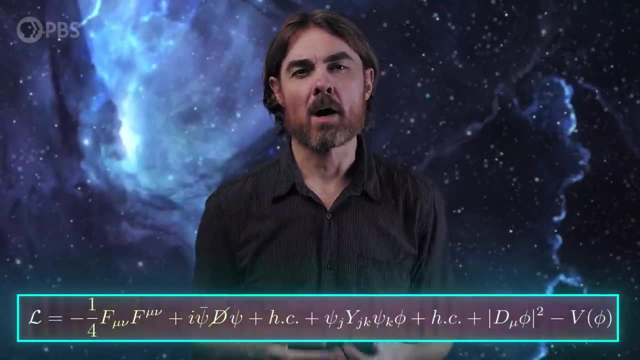 Well, hot coffee, because this is the point in reading the Lagrangian where most people need a coffee break. OK, bear with me, We're getting there. The particles described by the Lagrangian so far are massless. To add mass, we need the Higgs field. 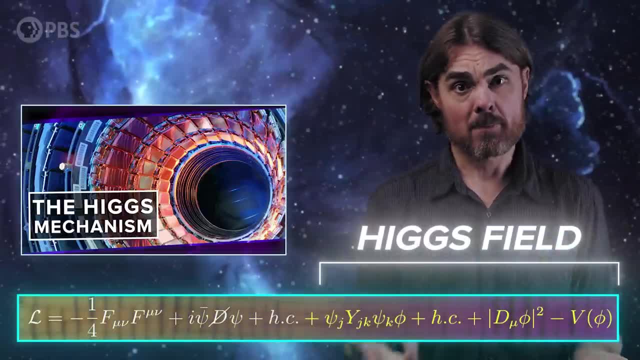 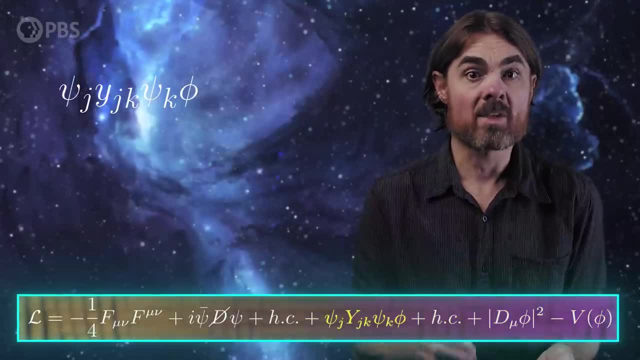 And that's what the rest of the Lagrangian deals with. We have episodes on the Higgs mechanism, if you're interested. This term is like the previous: We have fermions interacting with a bosonic field, But now that's the Higgs field. 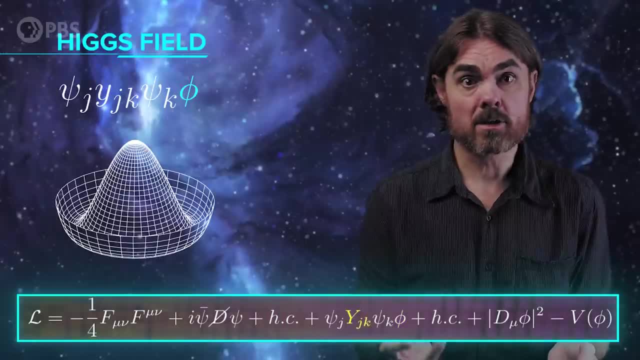 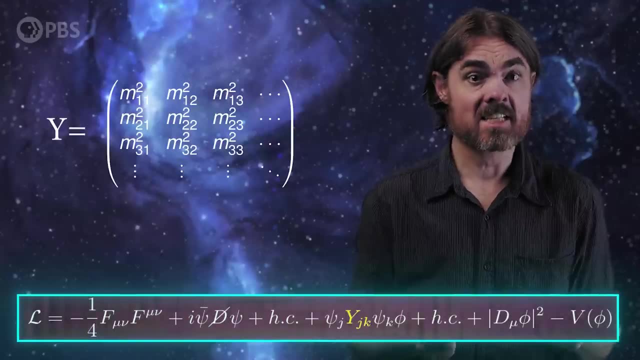 We have the Higgs field represented by this phi. Why is it a matrix with the square of the mass of each different fermion? This equation doesn't actually predict the particle masses. That's still an unsolved problem. Instead, we have to measure those masses with experiments. 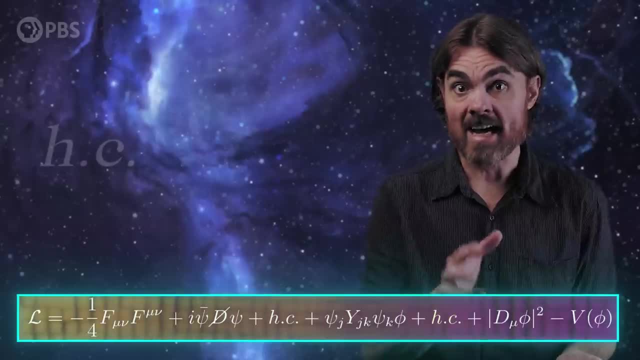 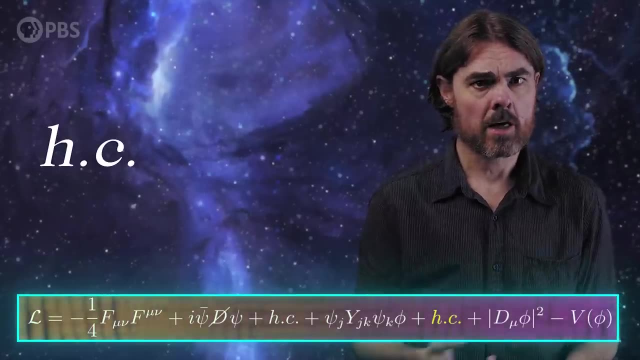 and then write them in this matrix by hand And we have another hc, But this time the permission conjugate tells us how antimatter picks up mass from the Higgs field, And it's pretty much the same way that the Higgs field does it, as far as we know. 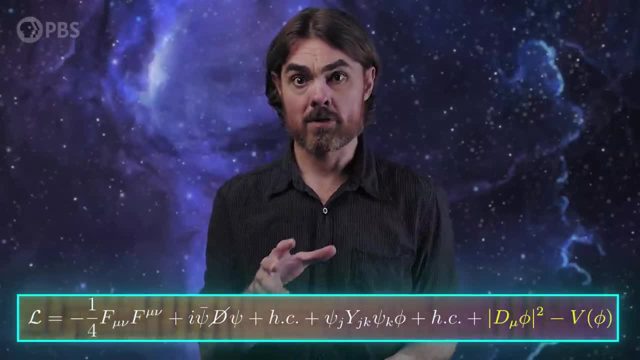 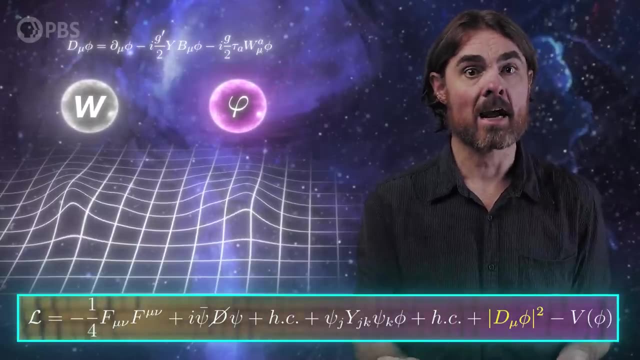 Let's zip through the rest of the Lagrangian. We have another one of these derivatives d, Now applied to the Higgs field. it tells us how that field changes in space and time and how it interacts with the massive bosons of the weak force. 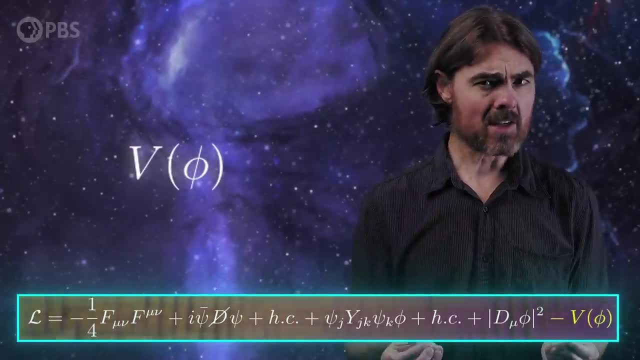 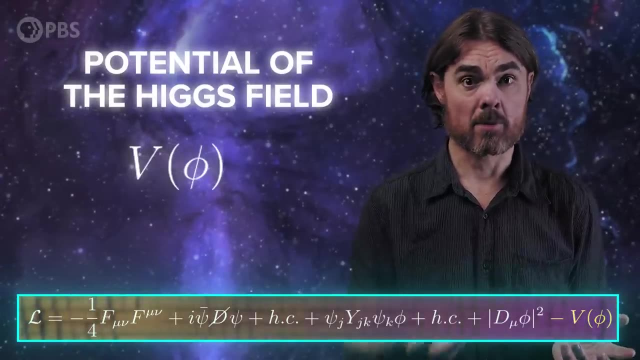 Finally, the last term refers to the potential of the Higgs field. This is like the kinetic term for the other bosons, but now just for the Higgs. The Higgs gets all its own terms, separate to the other bosons, which is quite special and weird. 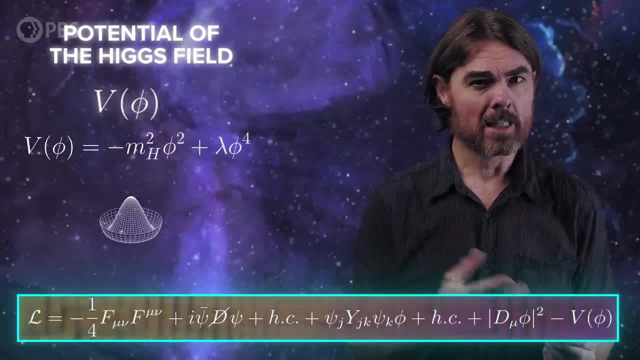 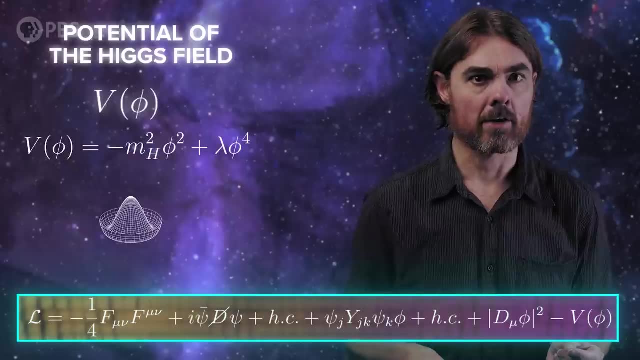 Really, though, this term describes the Higgs boson itself. That particle was the last prediction of the standard model to be verified, And that happened 10 years ago at the Large Hadron Collider. The discovery of the Higgs boson completed the standard model. 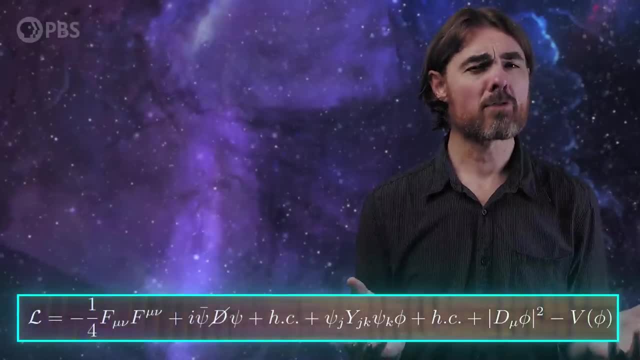 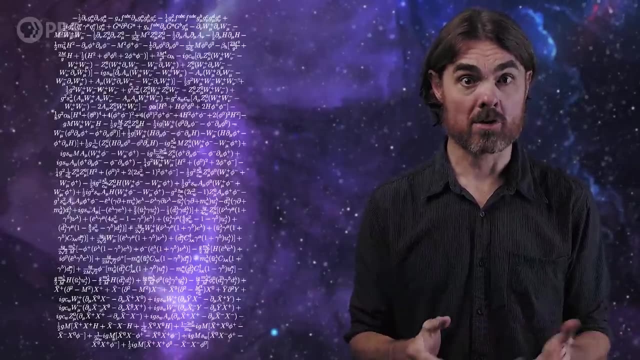 just as we finished the standard model Lagrangian, Now, just for fun, let's look at the full Lagrangian unsquished. Yeah, It's a lot, But that's not the reason why we're trying to come back to AI systems. 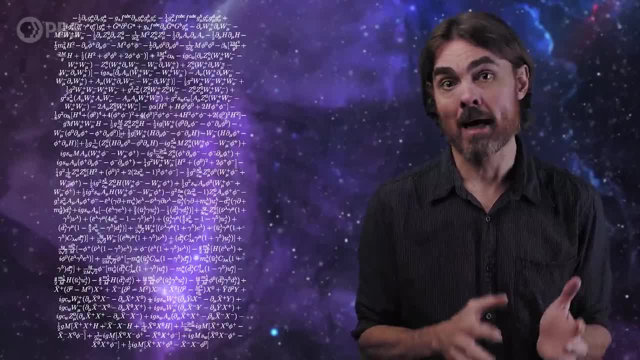 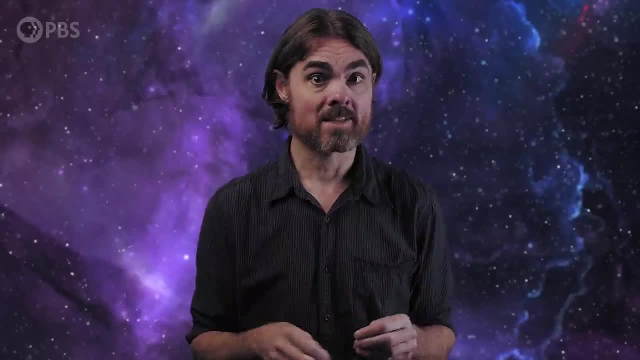 One way it works: Putting in your particle wave function and setting your indices right and including the correct masses, you can calculate the behavior of any known particle in the universe. Note, though, that I said known particle. There may be unknown particles that 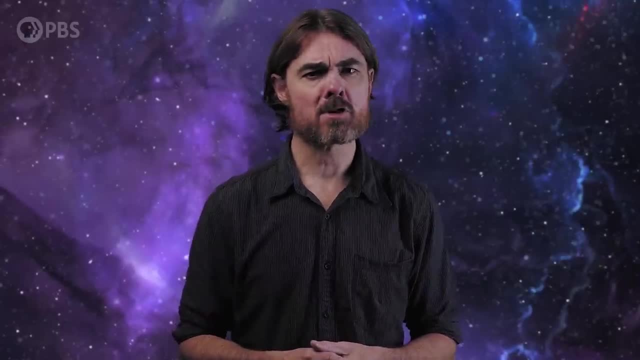 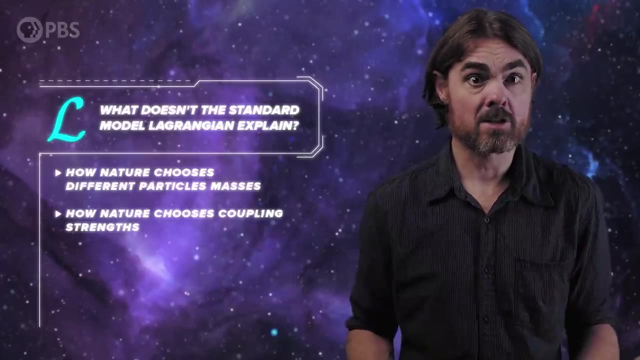 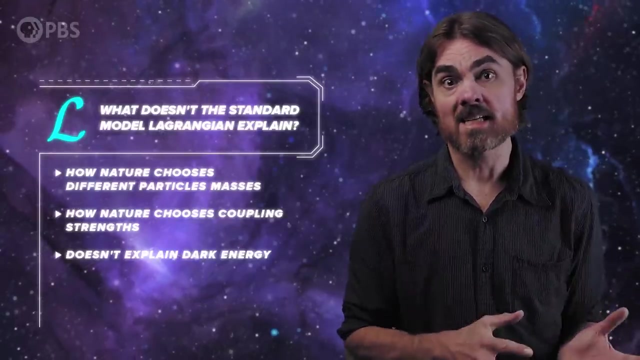 are not covered by the standard model or it's Lagrangian. In fact, there probably are Whatever makes up dark matter, for example masses, or chooses, coupling strengths, like the fine structure constant that we discussed recently, And it doesn't explain dark energy or the matter-antimatter imbalance, among other things. 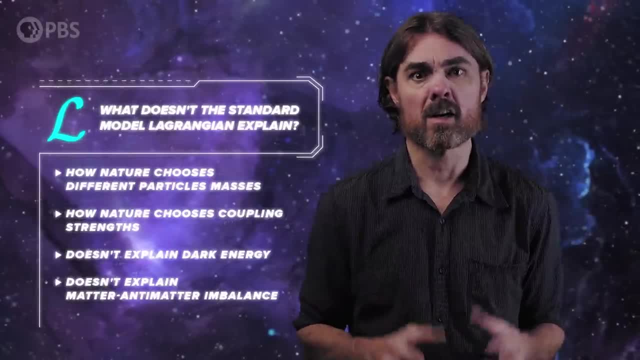 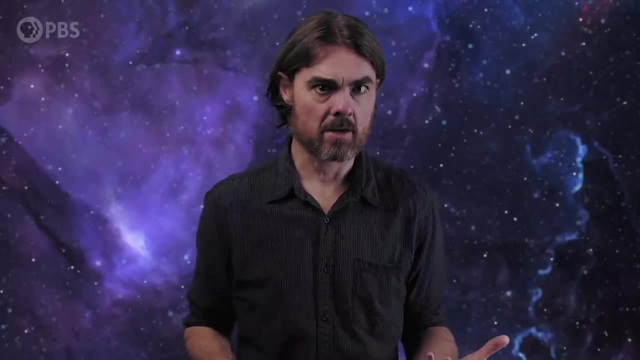 And it is a bit of a mess. Many physicists feel that the equation that truly underlies everything, if it exists, should be at least as elegant as E equals mc squared. But despite all of this, the standard model Lagrangian is an insane victory for physics. 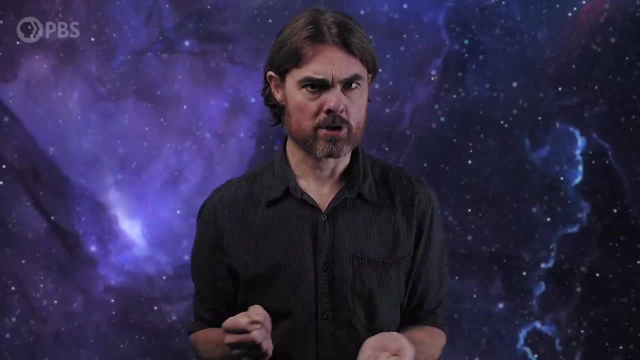 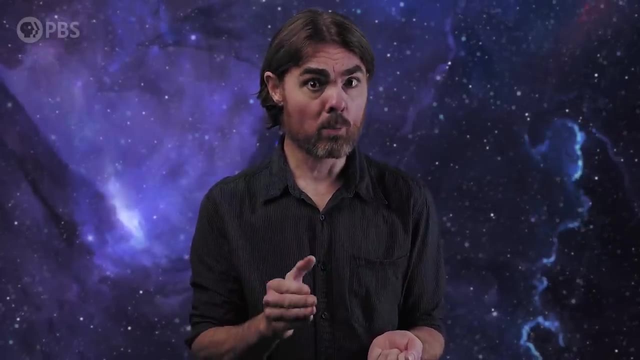 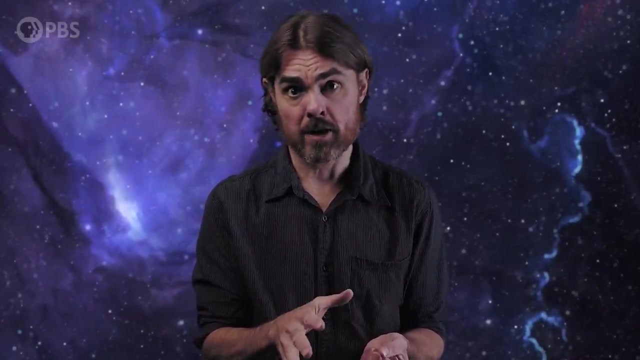 It predicts the behavior of the subatomic world with truly astonishing precision, And physicists are having a very difficult time finding situations where it fails, Because it will be a glitch in the predictions of the standard model Lagrangian. that could lead to an equation that is easier to fit on a coffee mug and to a deeper description. 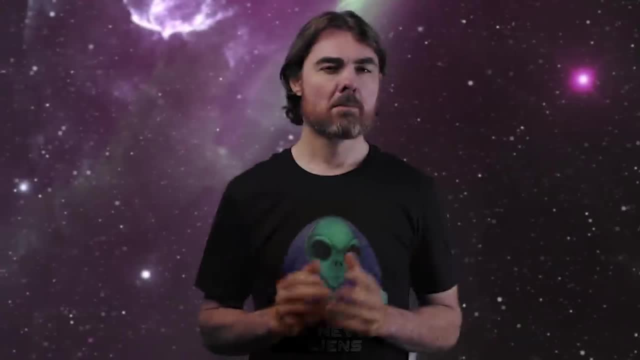 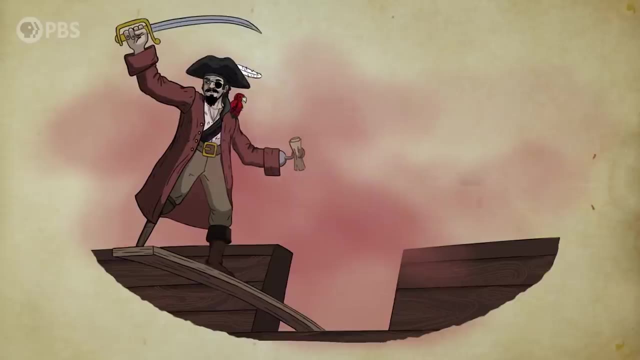 of the mechanisms ruling spacetime. Before we get to comments for all of the spacetime fans who are also history buffs, we'd like to let you know that we're going to be doing a lot of research on the space time. We're going to be talking about the new pirate-based history show called Rogue History. 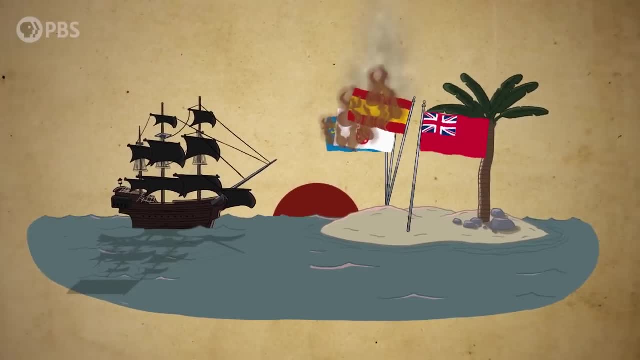 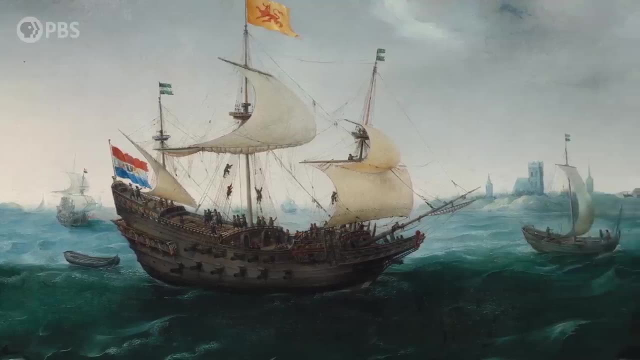 Over on the PBS Origins channel. Rogue History unravels the historical myths, unearths lost narratives and champions the unsung heroes of piracy. There's a link in the description and if you check it out, let them know politely that. 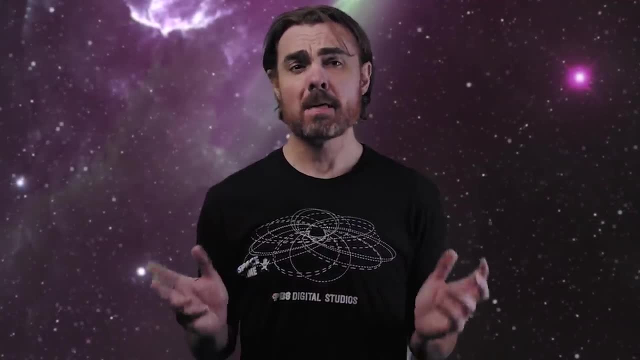 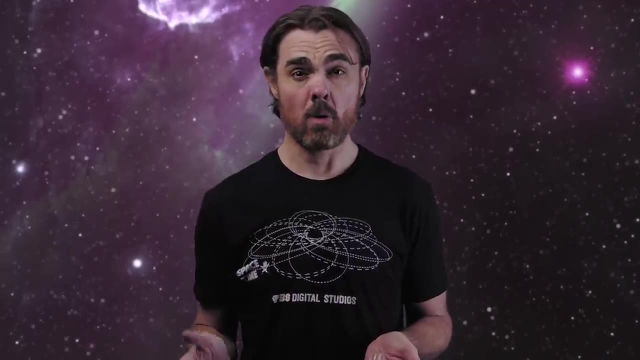 spacetime sent you. The support we get from Patreon is a big part of what makes this show possible, so thank you to everyone who donates Seriously. even a few bucks a month goes a long way, But today I'd like to give very special thanks to Vivan Guptavaka, who's supporting 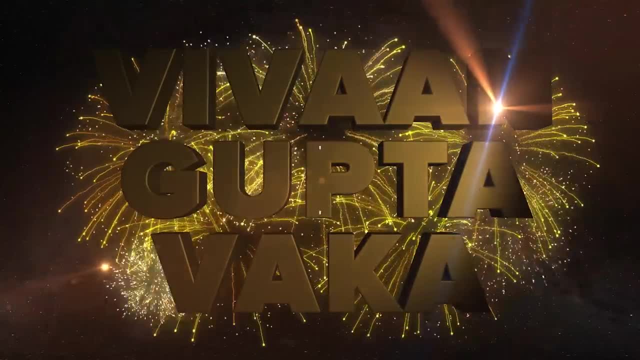 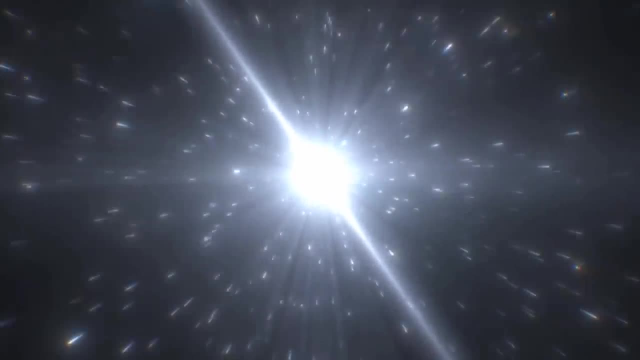 us at the Quasar level. For those of you who don't know, Quasars are the most brilliant objects in the universe. They are the hearts of galaxies, maelstroms of power and mystery shining out to us from across space and time.